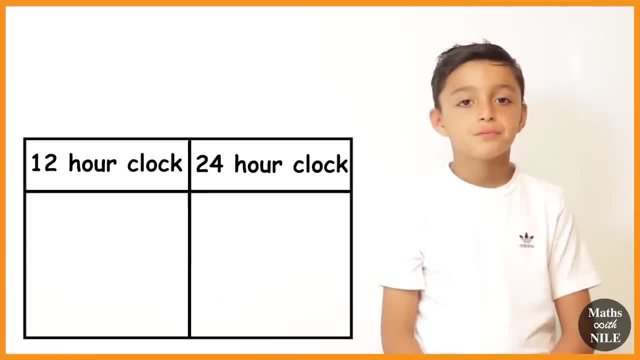 Okay. So how would you say two o'clock in the afternoon on a 12 hour clock, 2 pm, Very good. But when it's a 24 hour clock it's a bit different. How would you say two o'clock in the afternoon on a 24 hour clock? 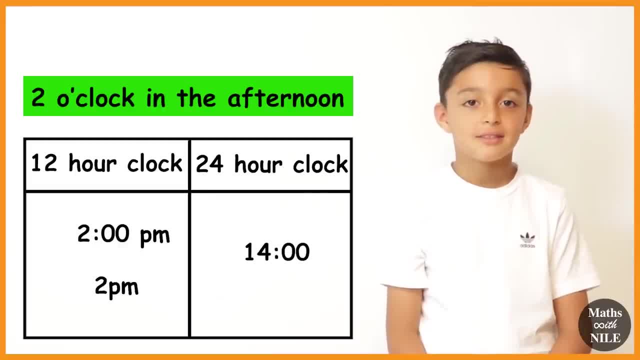 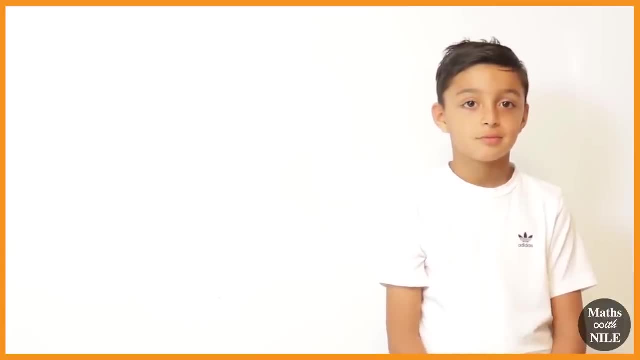 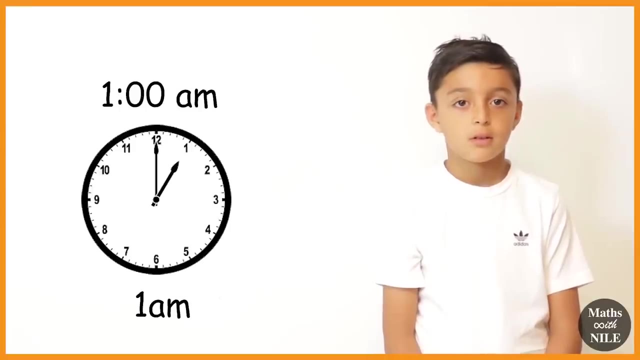 1400 hours. 1400 hours, So that sounds quite different to what we're used to, So let's have a look how it works. Can you go through the times from one o'clock in the morning on a 12 hour clock? So it starts at 1 am, 2 am, 3 am, 4 am, 5 am, 6 am, 7 am, 8 am, 9 am. 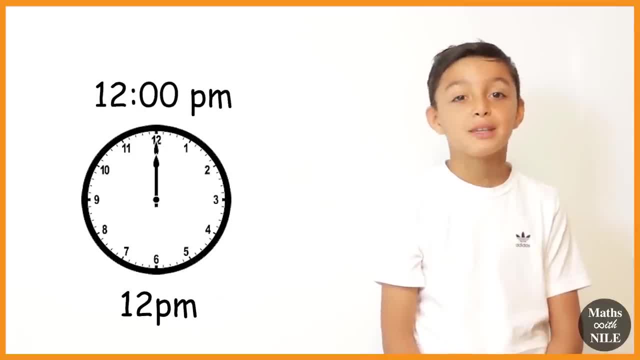 10 am, 11 am, 12 pm, 12 pm. And what happens at 12 pm? What time of the day is that? It's the afternoon, That's when midday is and that's when the afternoon starts, You're. 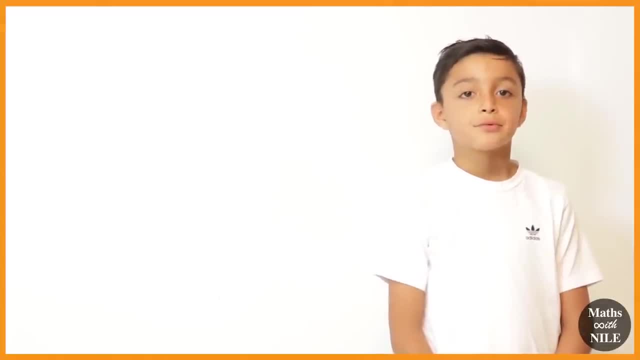 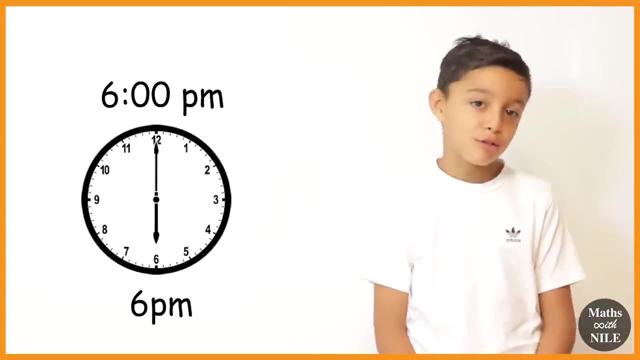 absolutely correct. So after 12 pm it goes to 1 pm, 2 pm, 3 pm, 4 pm, 5 pm, 6 pm, 7 pm, 8 pm, 9 pm, 10 pm, 10 pm, 11 pm, 12 am, 12 am. How else can we say 12 am? 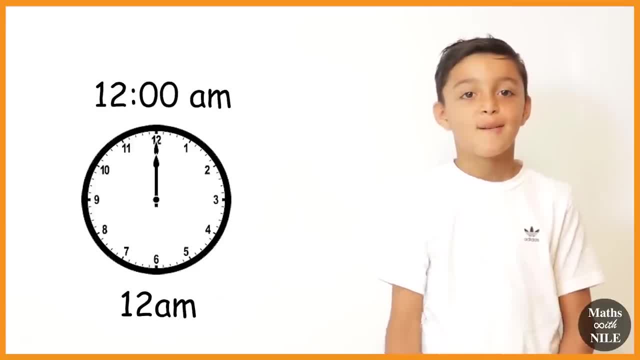 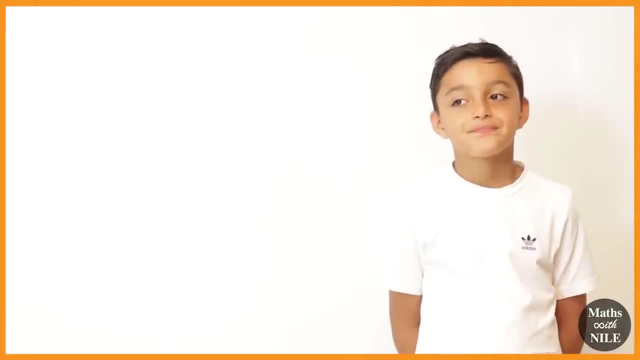 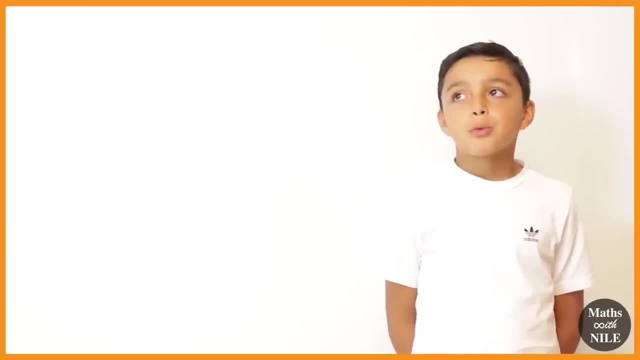 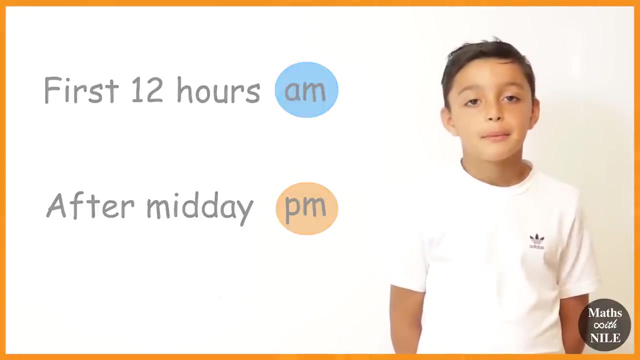 a 12 o'clock with am and pm. So we so the first 12 hours, you would say am, and then after 12 o'clock, which is midday, you would say pm. Okay, but you're using the same numbers, 1 to 12,. 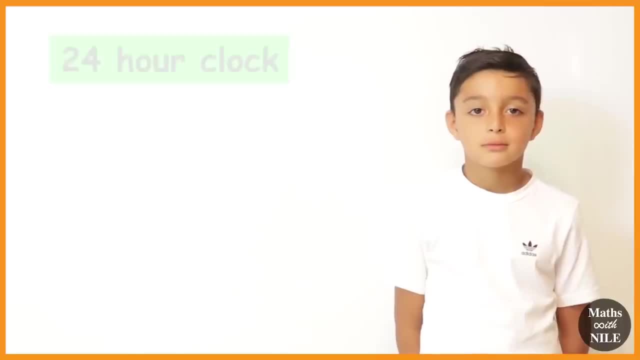 right, Yeah. So what happens when we do the 24 hour clock now? Do we use the numbers 1 to 12 or no? Um, no, we use um 1 to no, 0 to 23.. To 23? So don't we not use 24?? 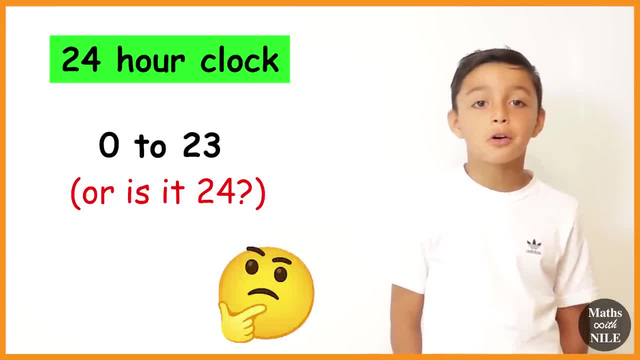 No, even though there are 24 hours in a clock, it's like minutes. there are only 59 minutes until the next hour. There are only 23 hours until the next day. Oh, can I tell you something quite interesting? What? 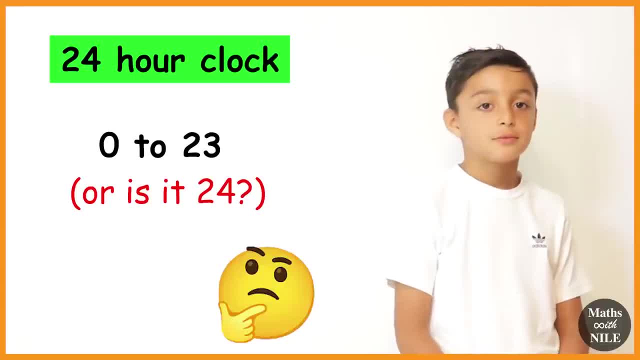 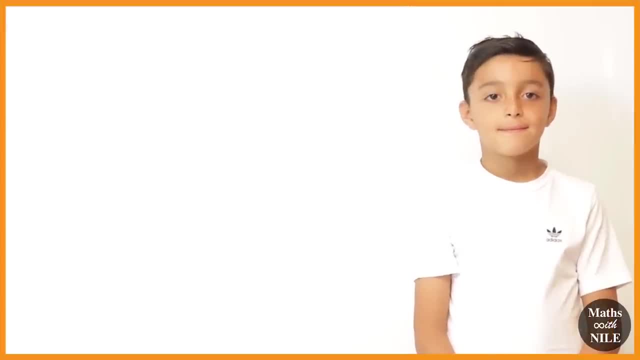 Some people do say 2400 hours. We'll have a look at that in a minute. Oh, do they? Yes, they do. Okay, now let's do some conversion from 12 hour to 24 hour. 5 o'clock in the morning. 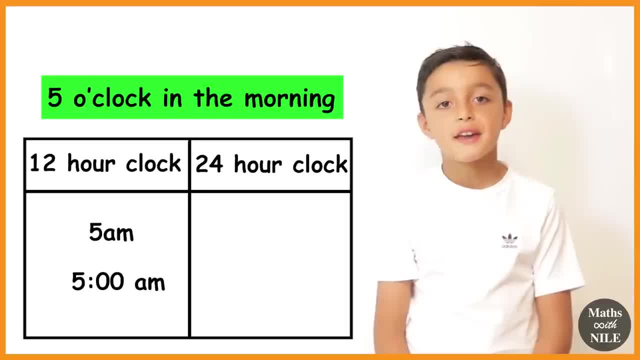 how do you say it on a 12 hour clock 5 am And how would you say 5 o'clock in the morning on a 24 hour clock 0 500 hours or 0 500 hours. Okay, so why did you put a zero in front of the five? 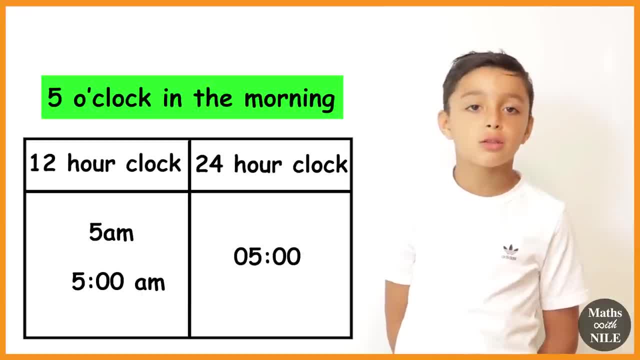 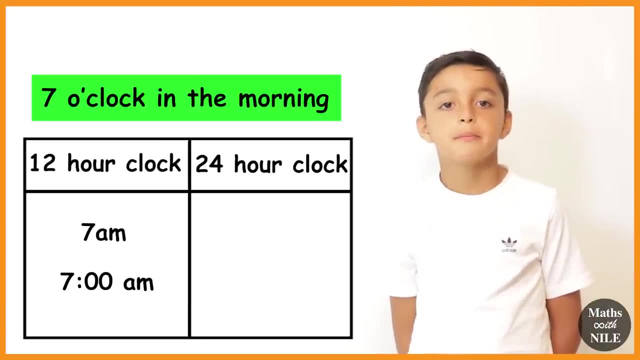 Um, because there always has to be two digits, um, when we're using a 24 hour clock, So we need to have two digits for the hours. is that correct? Yes, Okay, so how would you say 7 o'clock in the morning on a 12 hour clock? 7 am? 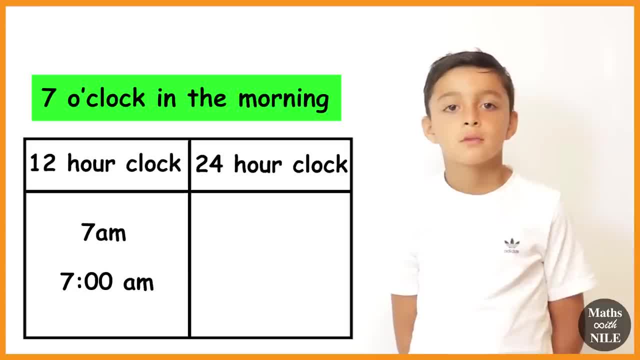 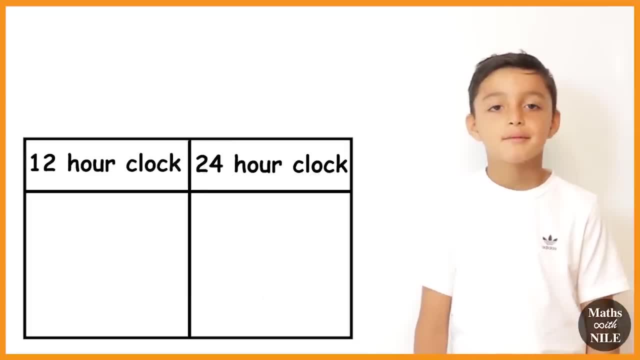 And how would you say 7 o'clock in the morning on a 24 hour clock, Um 0, 700 hours? Good. How would you say half past nine in the morning on a 12 hour clock- 9: 30 am? And how would you say half past nine in the morning on a 24 hour clock? 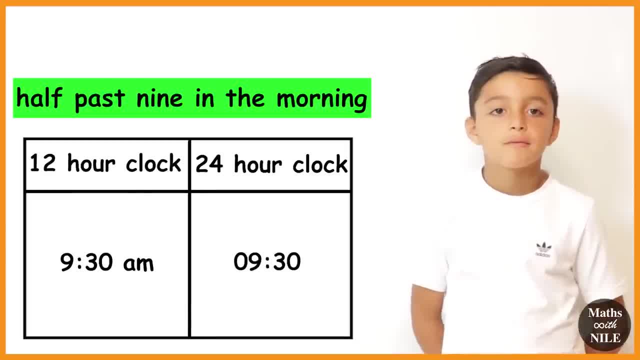 Oh 9, 30.. Oh, 9, 30. And what's in between the oh nine and the 30?? A colon, A colon. So we have the same colon that we use in the 12 hour clock. Dot dot. 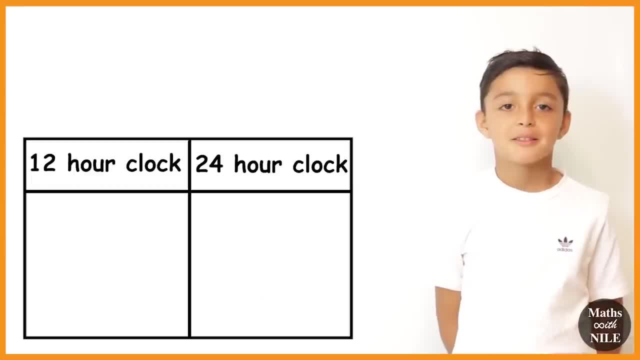 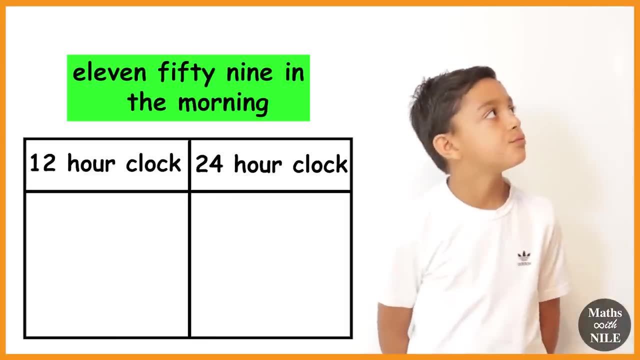 Correct. Okay, now it starts getting interesting when we get to midday. So how would you say 11: 59 in the morning on a 12 hour clock? 11 59 in the morning, 11 59 am, And how would you say it on a 24 hour clock? 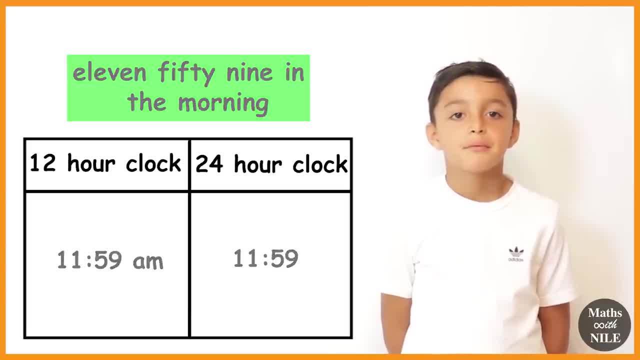 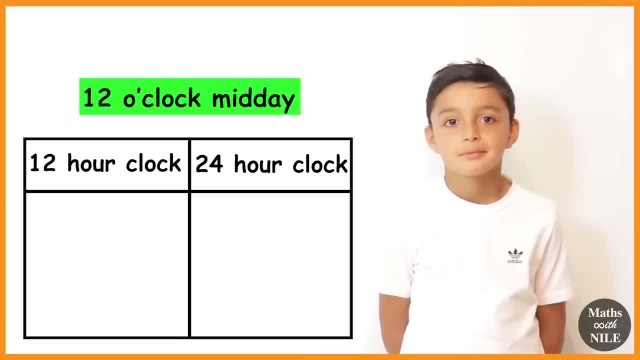 11, 59.. Good At 12 o'clock midday. how do you say it on a 12 hour clock? 12 pm, 12 pm, so that's when the afternoon starts right? Yes, and sometimes it can get confusing when like. 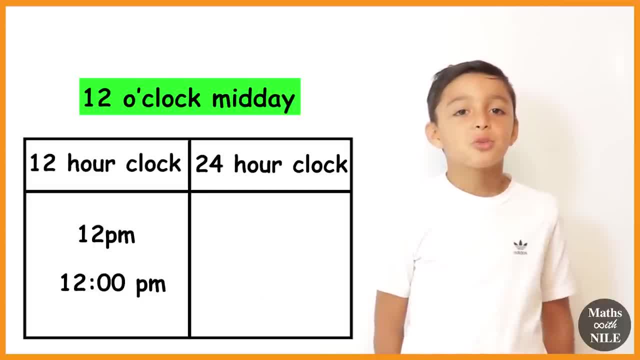 in a maths question and they put 12 pm. sometimes you would think it's midnight. can I tell you that another reason we use the 24-hour clock: so that we don't get the times between midday and midnight confused. yeah, okay, so you? 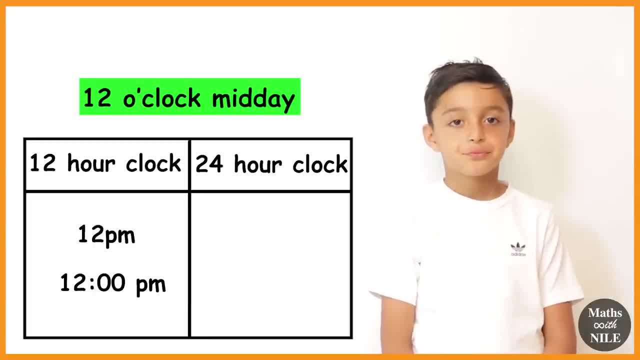 said midday is 12 pm on the 12-hour clock. what is it? only 24 o'clock, 1200 hours, brilliant. now we go on to 1 o'clock in the afternoon. so how do you say 1 o'clock in the afternoon on a 12-hour clock? 1 pm- good, but what? 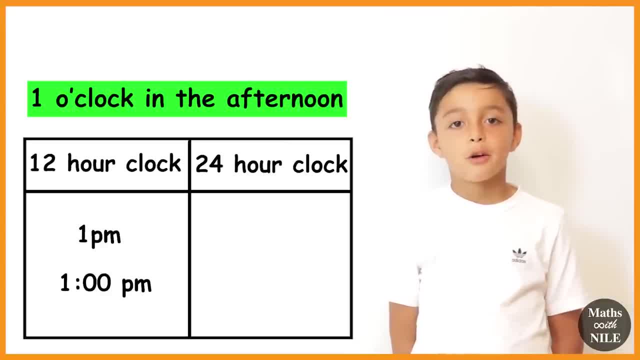 happens on the 24 o'clock now it goes over 12 and it turns into 13. so how do you say it? 1300 hours, 1300 hours and 2 o'clock in the afternoon. on a 24-hour clock it would be 1400 hours, 3 o'clock, 1500 hours, 4 o'clock, 1600 hours, 5 o'clock, 1700 hours. 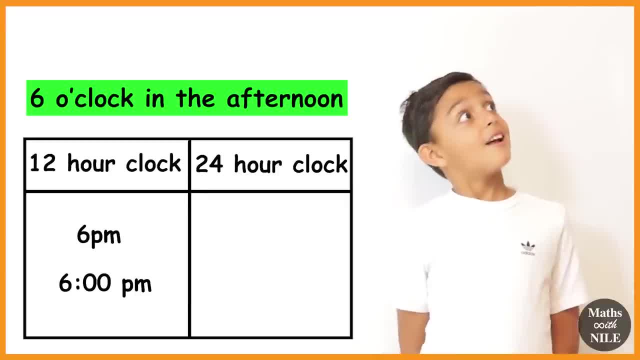 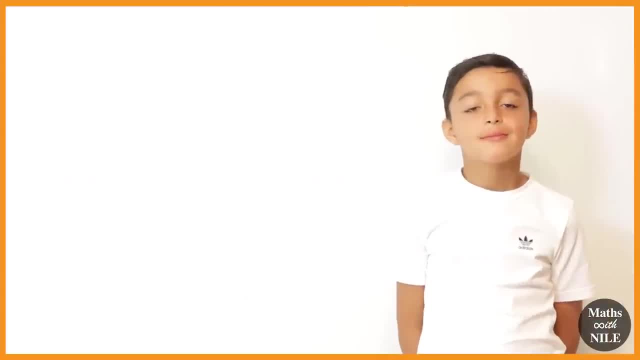 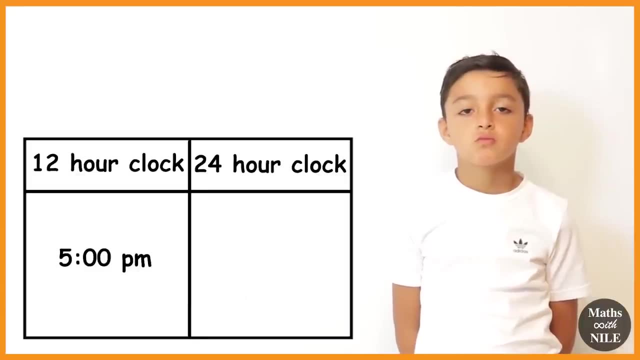 6 o'clock, 1800 hours, are you sure? okay, and it continues. okay, what's the fastest way to work it out? for example, if I wanted to know what 5 pm on a 24-hour clock is, what would you do? just add 12 and 5, and 12 is 17, so it would be 1700. 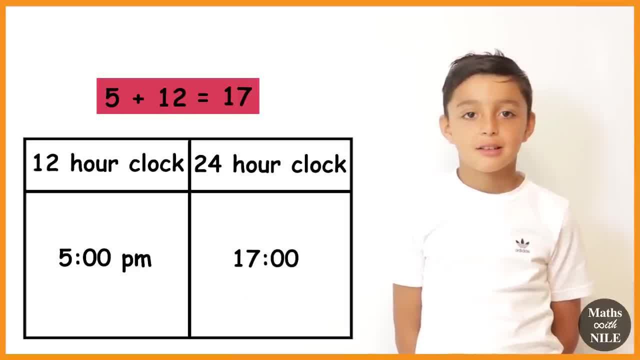 hours. brilliant, very, very simple. so if I said to you what is 8 PM on the 24 hour, clock 12 and 8 is 20, so it would be two hundred hours excellent. what about 11 pm on the 24 hours? 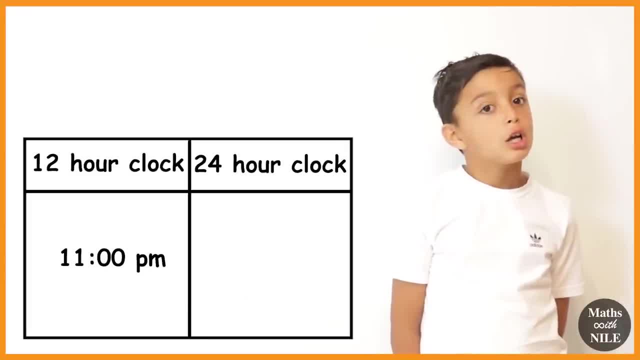 it would be what be? 2300 hours. Okay, Tash, share the calculation with us. So you would just add 12.. So 12 plus 11 is 23,, so 2300 hours. Yeah, It's very, very simple to change from 12 hour to 24 hour. 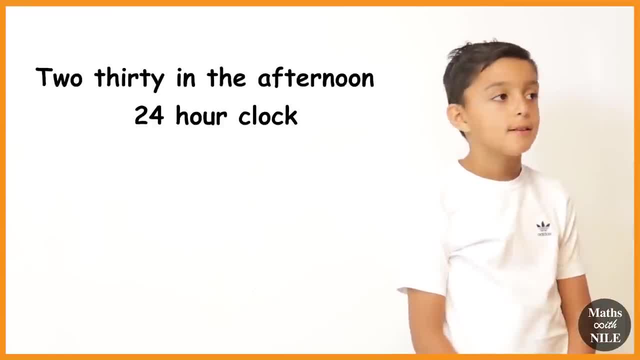 So how would you say 2.30 in the afternoon on a 24 hour clock? So you would do 2 and 12,, which is 14,, so it would be 14 and then 30,, so 14.30.. Very good, Niall, Very good. 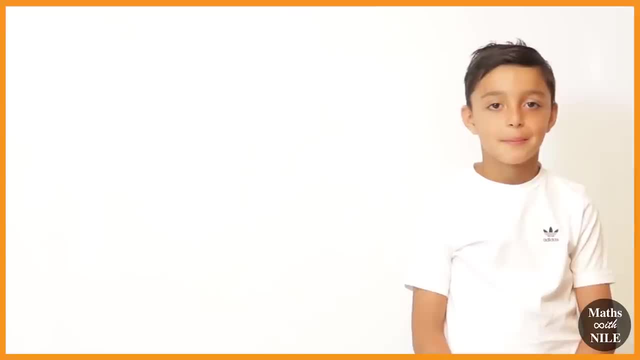 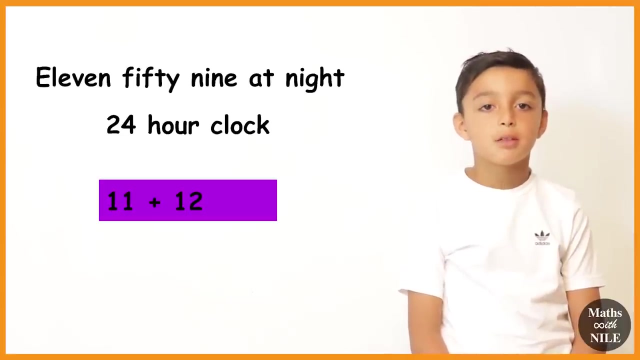 Now let's talk about when it starts getting towards midnight. So it is 11.59 at night. How do we write that on the 24 hour clock? So we do 11 plus 12, which is 23,, so it would. 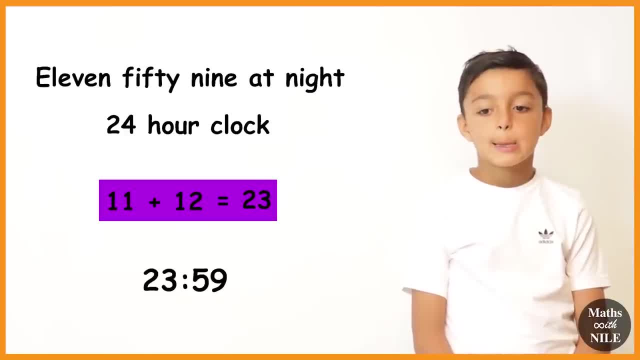 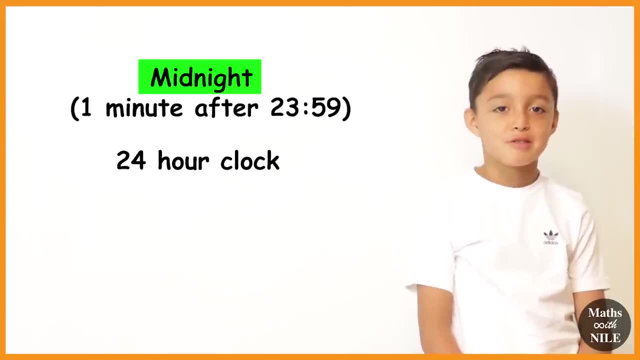 be 23.59.. Very good. And what happens when it gets to midnight, Niall? It becomes 0000.. So let's discuss that for a minute. It does, you're absolutely correct, because the next day is starting, Yeah, or has started. 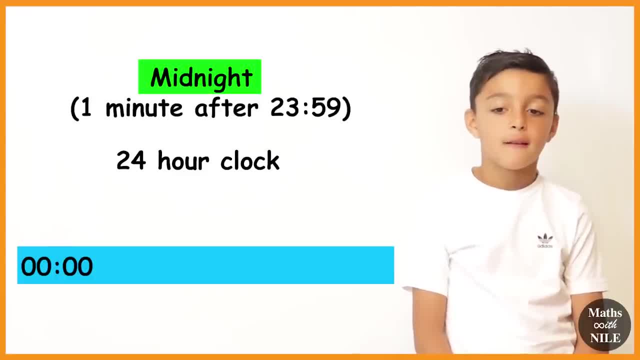 Yes, but isn't it also the end of the first day? Yeah, So can I just say to you that we can use 2400 hours to suggest that it's the end of the first day, Or we could do 0 o'clock. 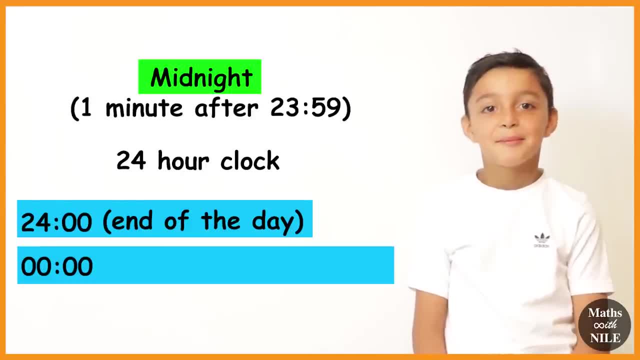 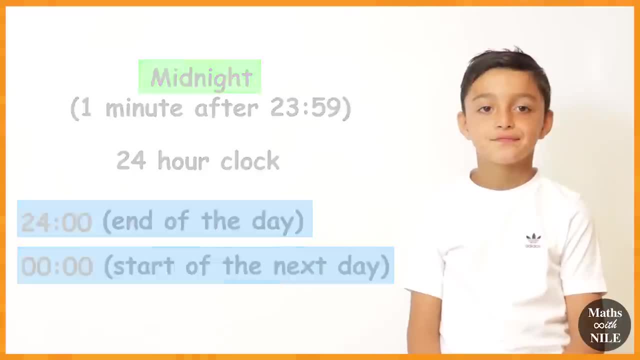 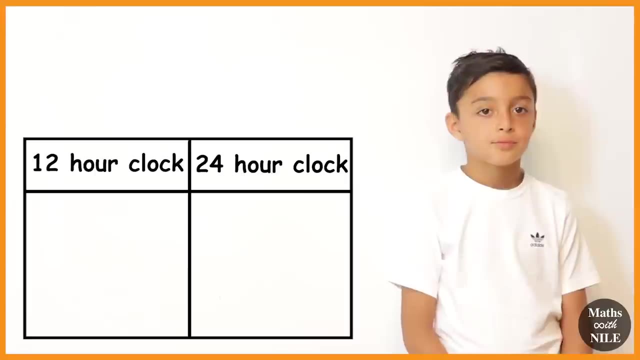 Or we can use 000 hours to say that it's the start of the next day. Yeah, so they're both correct. Okay, brilliant, Okay, Niall, what about if we were changing from 24 hours to 12 o'clock, For example, 1700 hours? What time is that, using the 12 o'clock 5pm And? 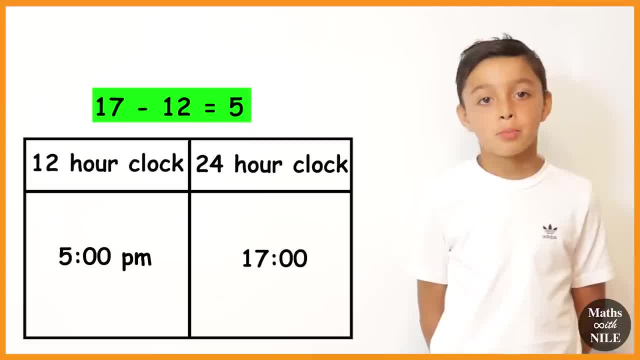 so basically, you just take away 12 and then add am or pm. if you're changing it to a 12 hour clock, Okay, so you've done 17,. take away 12.. And then put am or pm: Okay, and how do you know it's pm If it's in the afternoon? Okay, so you've done 17,. take away 12. And 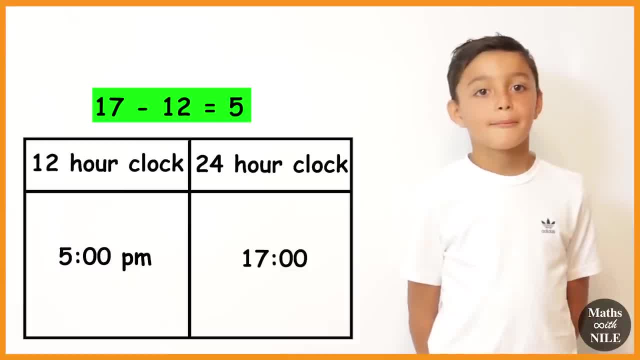 then put am or pm. Okay, and how do you know it's pm If it's in the afternoon? Okay, so you've done 17,. take away 12.. Okay, because it's gone past 1300 hours. So that's when. 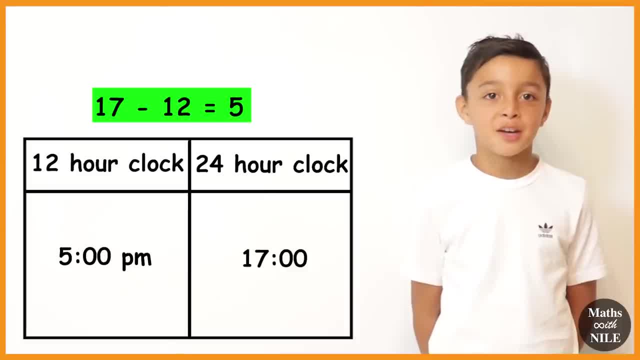 we know we're in the afternoon. Well, actually 1200 hours. Very good, Good correction. Thank you, Niall. What would 1900 hours be? on the 12 hour clock, Niall, 1900 hours would be. 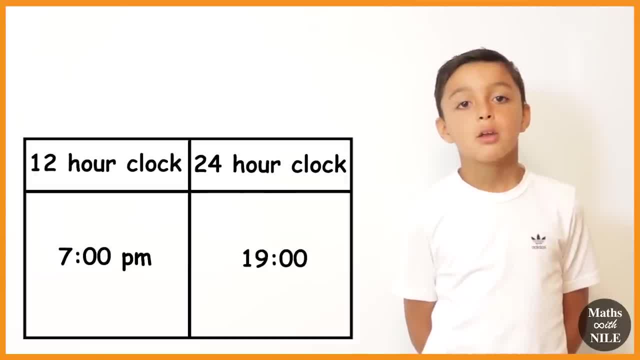 7pm, And because 19 is past the 1200 hours, it would be in the afternoon, And if it's in the afternoon, on the 12 hour clock we would put pm and I took away 12.. You took away 12 from what? From 19.. That's why you got 7pm. Yeah, I got 7.. Okay, so can we do? 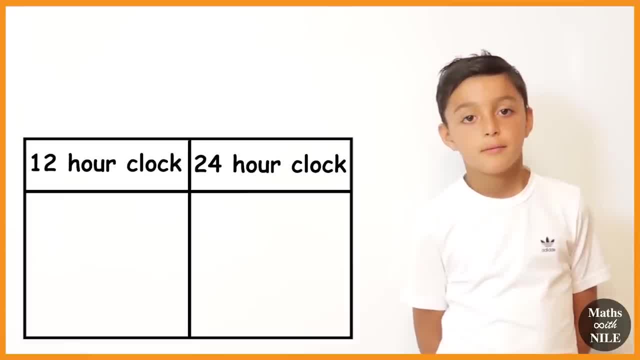 one more of those. Okay, 2200 hours. can you change that to 12 hour clock? That will be 10pm And so we do 22, take away 12, which is 10.. And then we put pm because it's past 1200 hours. Very, 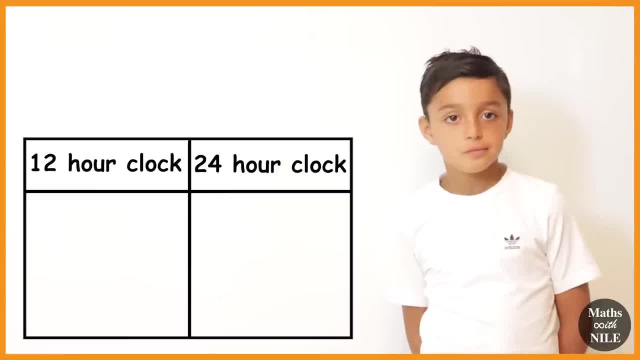 good. So what is 0700 hours in the 12 hour clock? 0700 hours, That will be 7am. I just got the 7 and put it, turned it into am and because it's not past the 12.. So what's the? 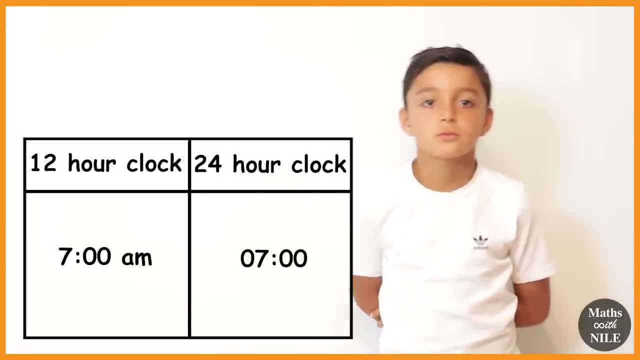 difference with the am on the 12 hour clock compared to 24 hour clock. So let's look at the time 7 o'clock in the morning. What's the main difference? You would put am on the 12 hour clock and you wouldn't on the 24 hour clock. And there's something else we would. 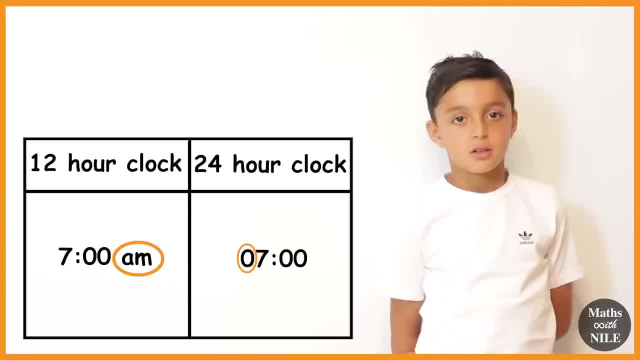 do on the 24 hour clock. You would put a zero in front. That's it, So the time is 7am. And you would put a zero in front. And you would put a zero in front, That's it, So the time. 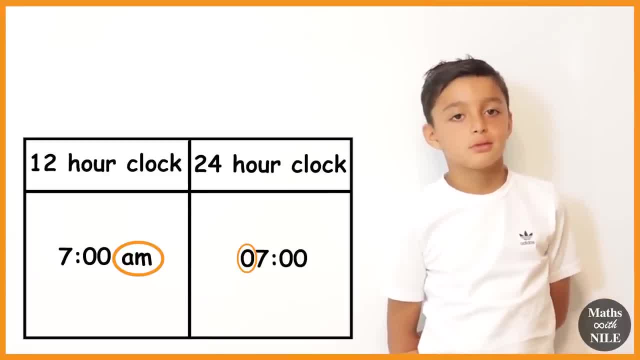 when it's am, it looks the same, apart from not having the am when, if it's 24 hour, and not having a zero if it's 12 hour. Yeah, Very good, Niall. One last benefit, Niall, of the. 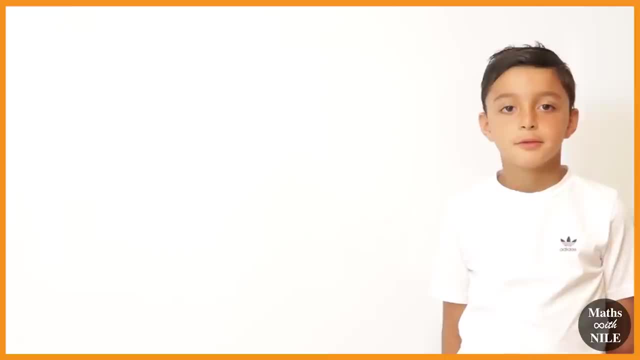 24 hour clock. We can work out the difference between times very easily. For example, if I say to you how many hours between 10 hundred hours and 13 hundred hours, Um, 3. Because you can just take away 10 from 13 and it's 3.. Yeah, So what's the difference? 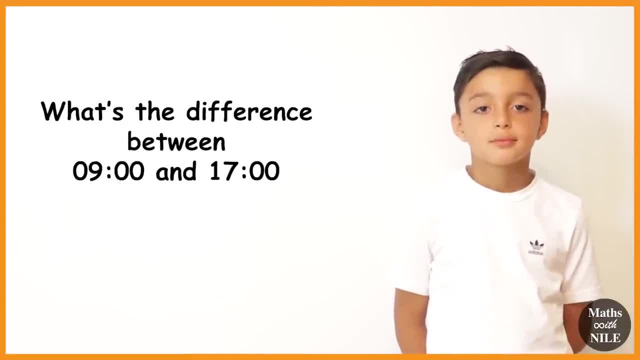 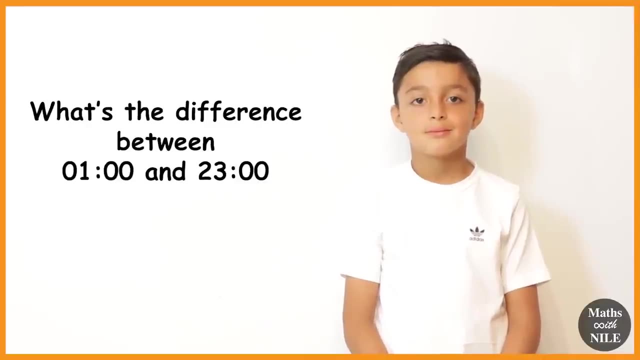 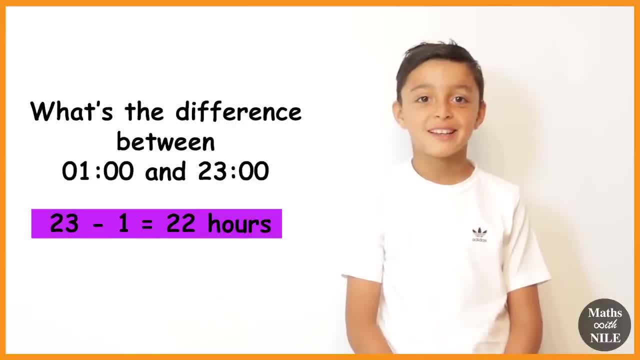 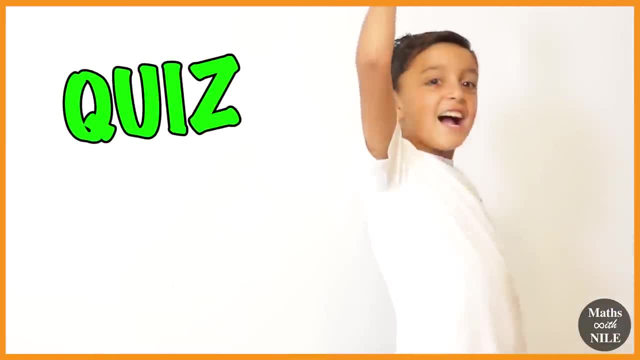 out. I just took away 1 from 23. Which is 22. So that's quite easy. Are you ready for the quiz? Oh yeah, Okay, 5 o'clock in the morning, 12 hour o'clock Um, 5 o'clock in. 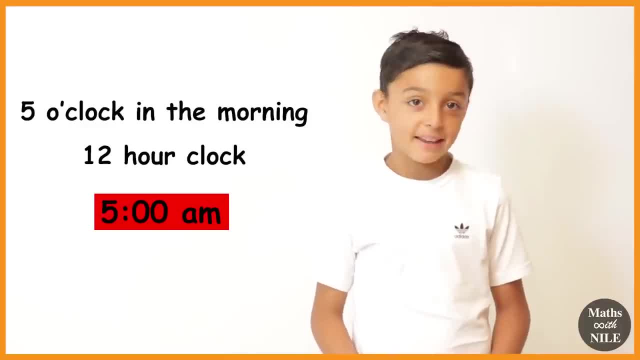 the morning 12 hour o'clock Ha. 5am 2 o'clock in the afternoon. 24 hour clock: 14 hours and 16 minutes. Um. 14 hours and 16 minutes. Ok, So it's a 12 hour clock time somewhere. 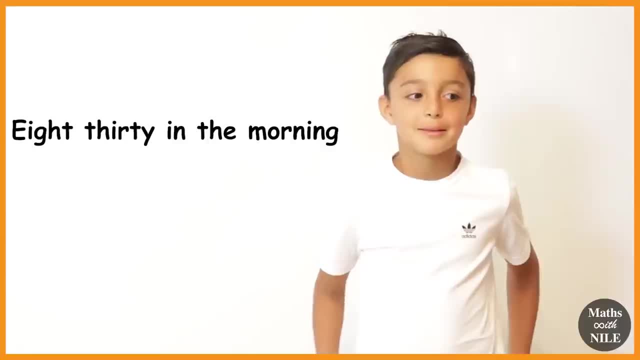 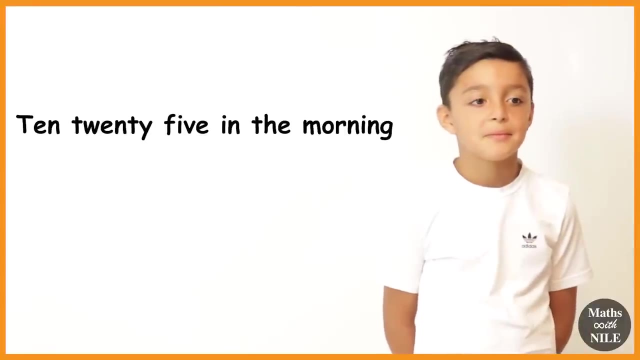 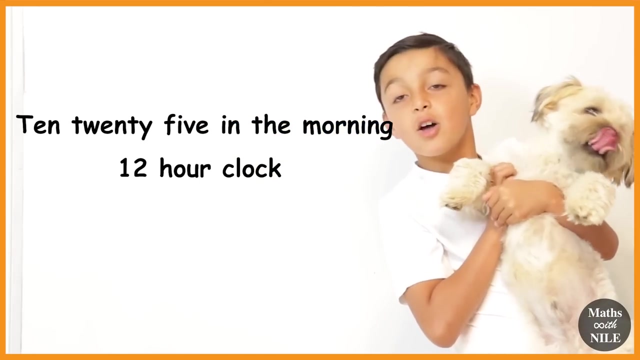 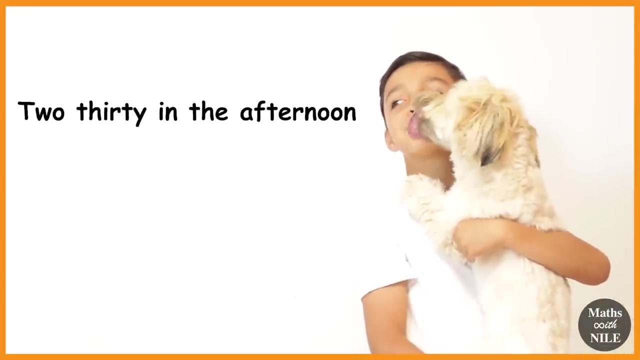 fourteen hundred hours okay: 830 in the morning, 12 o'clock, 830 am, 1025 in the morning, 12 o'clock, 1025 am, 2: 30 in the afternoon, 12 o'clock, 2: 30 pm, 4 o'clock. 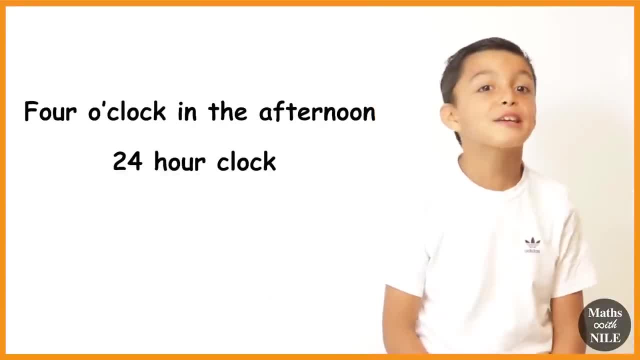 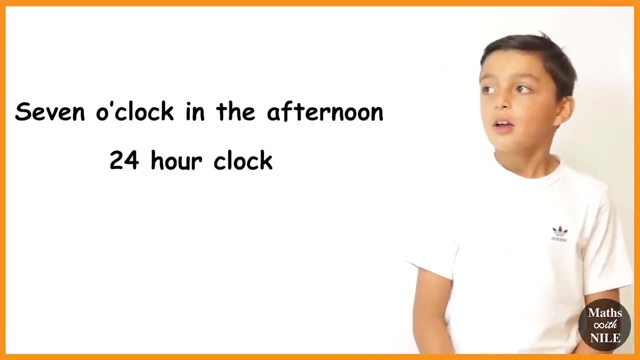 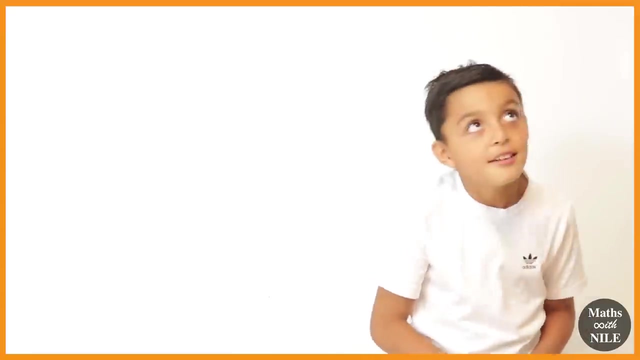 in the afternoon, 24 o'clock for 16 pm, 1600 hours. let me see it again: 4 o'clock in the afternoon, 24 o'clock, 1600 hours. 7 o'clock in the afternoon, 24 o'clock, 1900 hours. how do you see midnight, 24 o'clock, um 2400 hours, or? 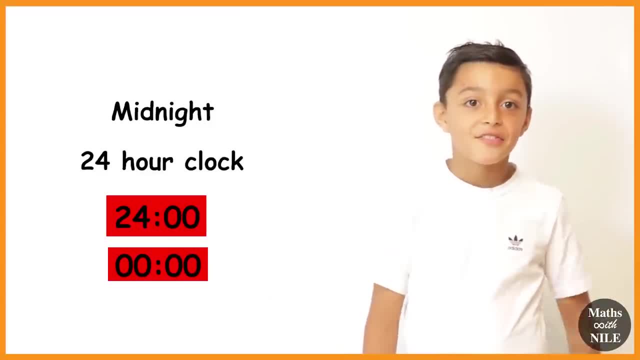 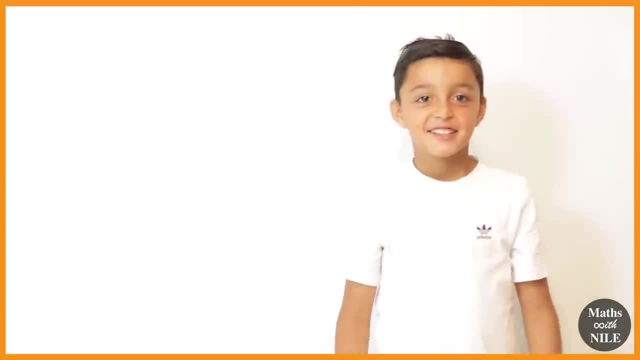 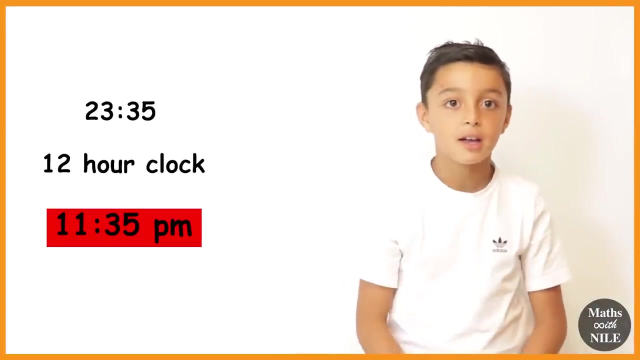 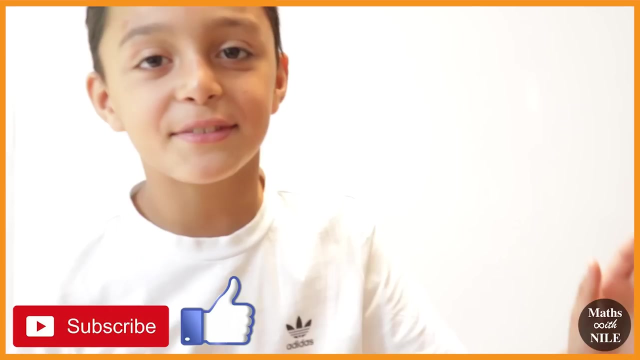 zero hundred hours. very good night, remember that. one last question: what is 2335 in the 12 hour clock? 23 um 11, 35 pm. very good night, and that comes to the end of today's lesson. bye, hope you enjoyed the video and, if you did, subscribe now behind the screen and leave a like on this video. bye.